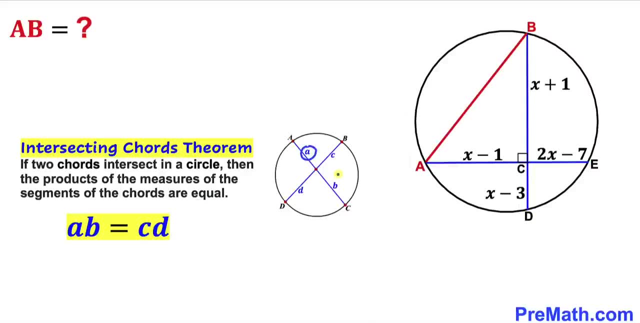 We can see the product of these two segments, a times b, equal to c times d, as you can see in this diagram. So therefore, let me go ahead and label this segment as lowercase a, this segment lowercase b, this c and this d. Let's go ahead and fill in the blanks in this formula. In our case, a is x minus 1 times b is 2x minus 7 equals to c. in our case is x plus 1.. 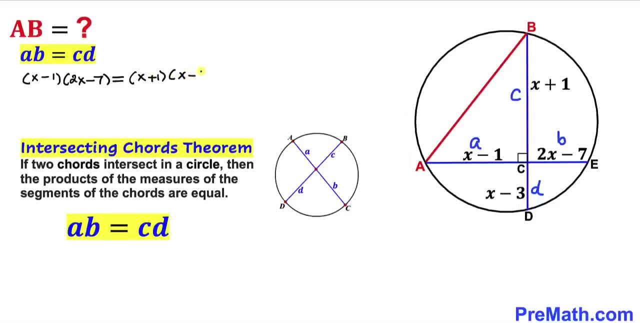 Let's go ahead and multiply these factors by double distribution, by just simply multiplying. Likewise, I'm going to do the same thing over here. Therefore, on the left hand side, we are going to get 2x squared minus 7 x minus 2x plus 7 equals to. on the right hand side, We are going to get 6 divided by 1.. So again, we are going to do the same thing over here. So therefore, on the left hand side, we are going to get 2x squared minus 7, x minus 2x plus 7 equals to: on the right hand side, 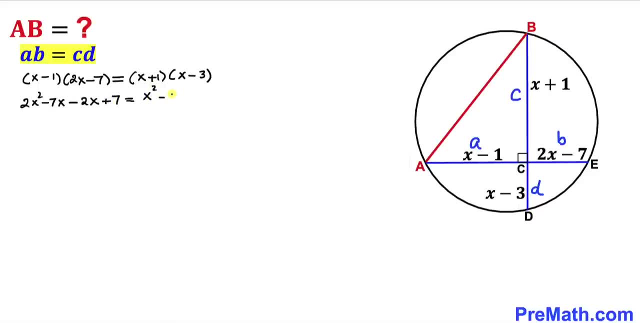 that's going to give us a x square minus 3x plus x minus 3. let's go ahead and combine the like terms on both side, so we are going to get 2x square minus 9x plus 7, equal to x square minus 2x minus 3. now let's go ahead and move everything. 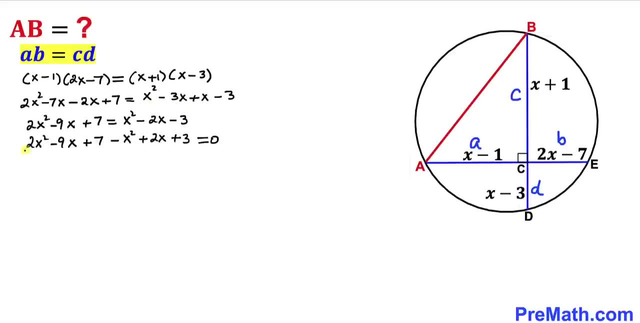 to the left hand side. let's combine once again, so that is going to give us x square minus 7x plus 10, equal to 0, and now we can see that we have x square minus 6x plus. all right, so let's go ahead and 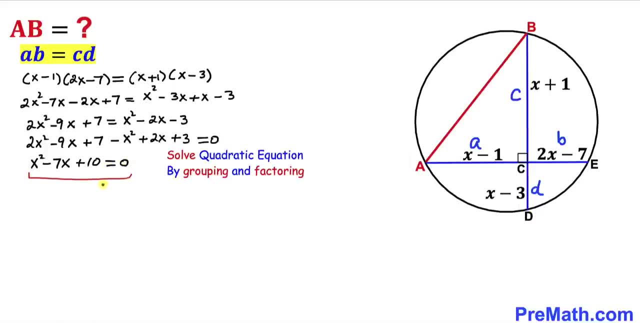 see that this is our quadratic equation and we are going to solve it by grouping and factoring, so therefore, let's focus on this negative 7x. this could be written as a negative 2x minus 5x, isn't it? so therefore, this is going to become x square minus 2x minus 5x plus 10 equals to zero, and here, 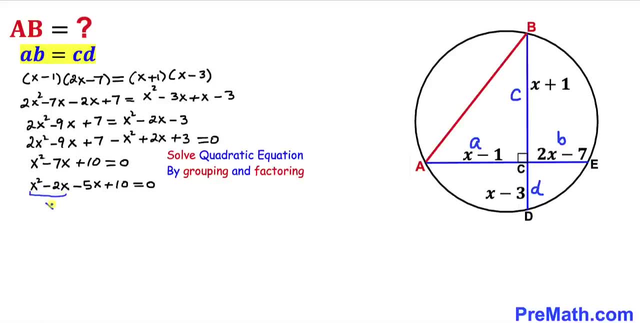 we can see between first these two terms, x is in common, and likewise in second two terms over here, negative of five is in common. so therefore we are going to write down x times x, x minus 2, minus 5, times x minus 2 as well, equal to 0, and here we can see x minus 2 and x minus 2. 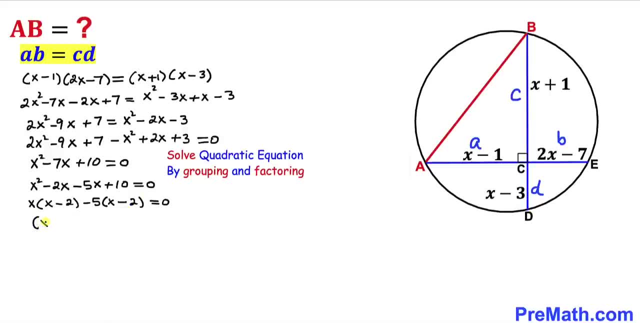 they are in common. so therefore we can write this thing: x minus 2 times x minus 5 equal to 0. now we got two factors equal to 0. let's go and separate them. I can write x minus 2 equal to 0, and the. 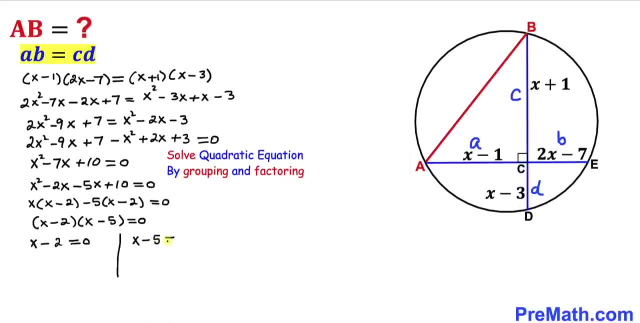 second factor: x minus 5 equal to 0 as well. now let's focus on this first equation: x minus 2 equal to 0 means x equals to 2 value. and for this second equation, x minus 5 equal to 0, x minus 2 equals to 0. and for this second equation, x minus 5 equal to 0. and for this second equation: 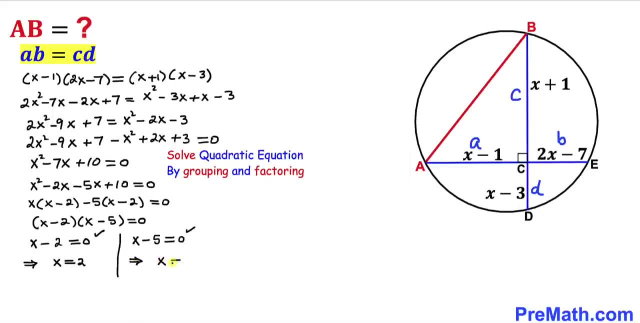 means our x value is going to be positive 5, and now we can see we got two values of x. let's focus on x equal to 2 value. if we plug it in over here, let's suppose on this one. so that is going to become 2 minus 3. that is going to be negative 1 and this represents the side length. so this cannot. 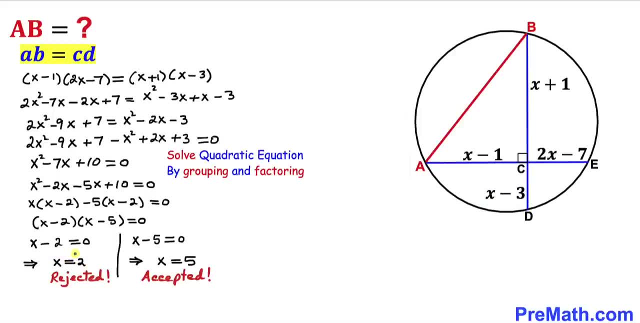 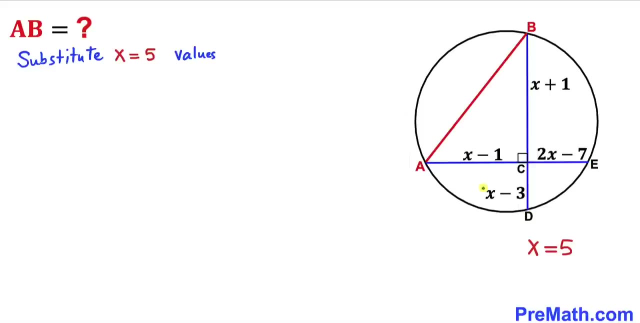 be negative. so therefore, we can see that x equal to 2 is not possible. no wonder we are going to reject this value and we are going to accept x equal to 5 value. and here's our next step. let's go ahead and substitute x equal to 5 values in these expressions, all of them, if we replace this. 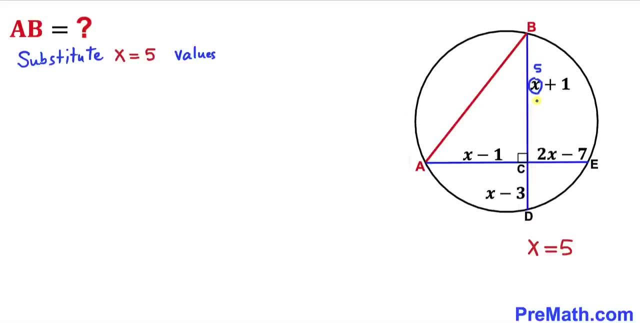 x by 5, so this is going to become 5 plus 1 is 6. and likewise, if we replace this x by 5, so that's going to give us 5 minus 1 is 4. and if we replace x by 5 over here, that is going to give us 3 value. and finally, if we replace this: 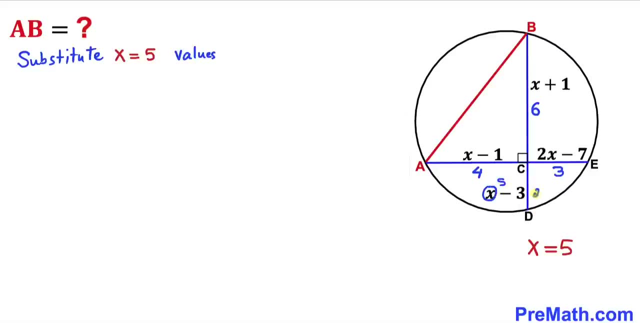 x by 5. that is going to give us value 2. and here's our final step. let's go ahead and calculate the length of this ab, and now let's focus on this right triangle, acb. so therefore, we are going to use the pythagorean. 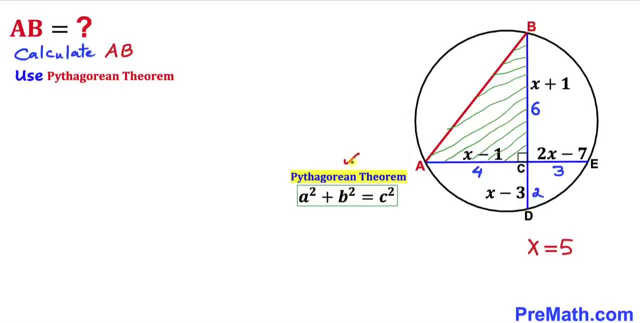 theorem, and here's our pythagorean theorem: a square plus b square equal to c square. let me go ahead and represent this longest leg as our side c. i'm going to call this side a and this side lowercase b. let's go ahead and fill in the blanks in this pythagorean formula: a, in our case, is a, 4. 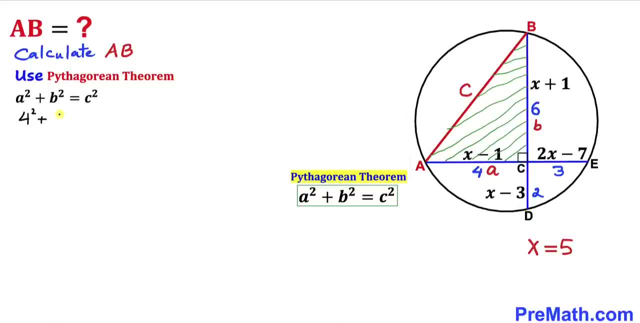 so this is going to become a 4, and this is going to become a 4 and this is going to become a 4, so this is going to become 4. square b in our case is 6, so 6 square equal to c square. so that's going. 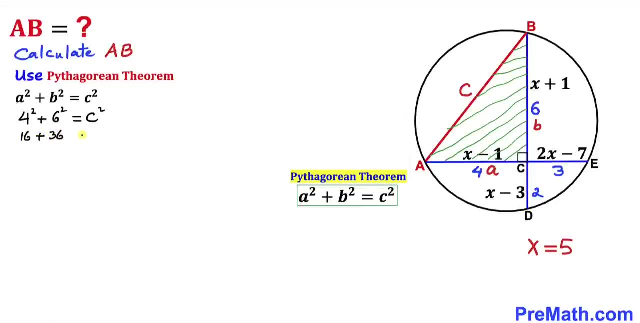 to give us 16 plus 36, equal to c square. so therefore c square turns out to be 52. let's go ahead and take the square root on both side to undo this square. this is gone. so therefore, c value turns out to be square root of 52, and now we can see square root of 52 could be simplified to 2 times.